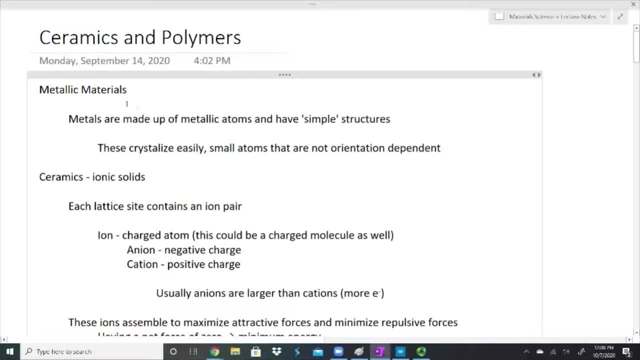 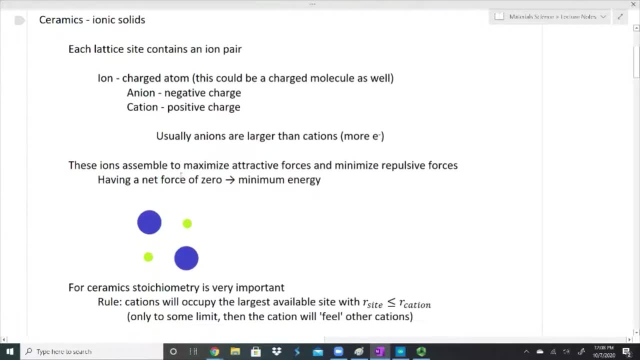 if we understand crystals, then we're going to understand much about metallic materials. right now We're going to jump into ceramics. We're going to go through these pretty quickly. This isn't meant to be a full discourse On all these. there are actually whole classes that you can talk about: ceramics and polymers. 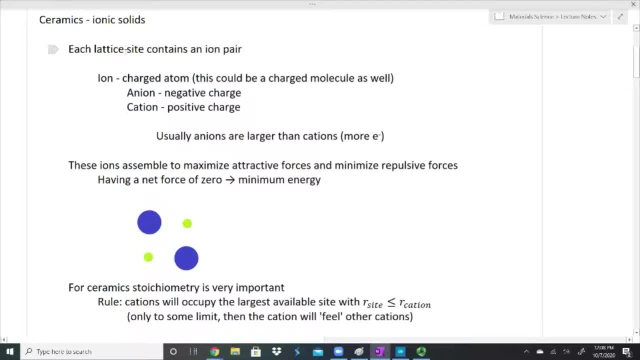 in Ceramics are also called ionic solids. In this case, for ceramics, each lattice site contains a pair of ions, not just a single atom, like a metal would. An ion is a charged atom. We have positively charged and negatively charged, namely anions and cations Usually. 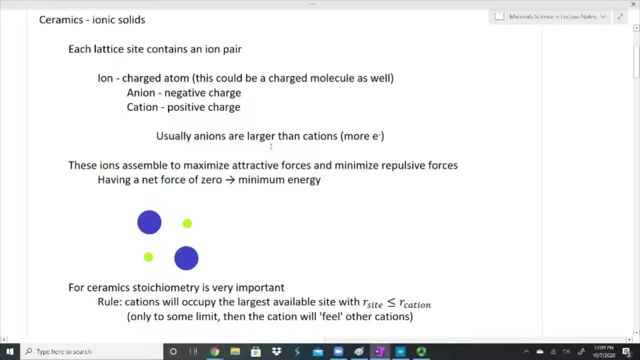 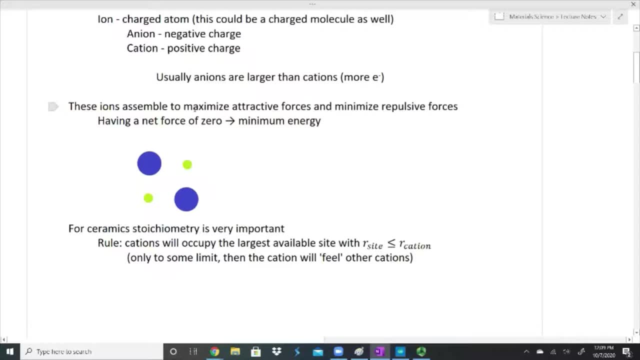 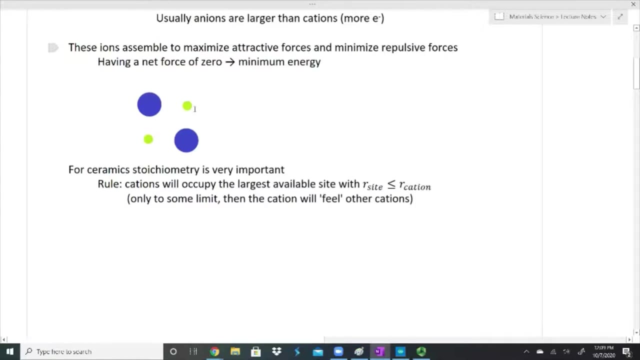 anions are larger than the cations and that's because there are more electrons. These ions are going to assemble to maximize the attractive forces and minimize repulsive forces. We talked about that when we discussed bonding. What we want to do is we want to get into a little bit of stoichiometry. That's a very 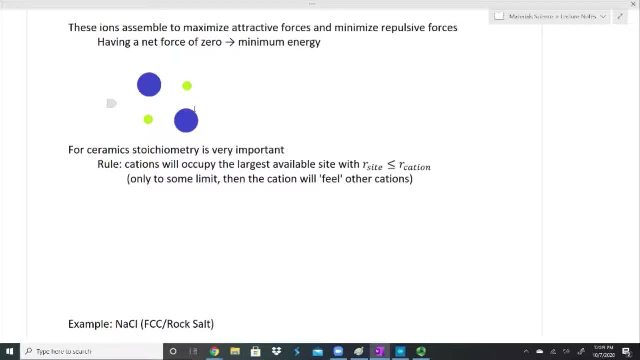 very important part of stoichiometry. Okay, Okay, Ceramics. we're not going to get into it a whole lot, but what we need to do is we need to just make sure that our picture, or that the anions and the cations that we're 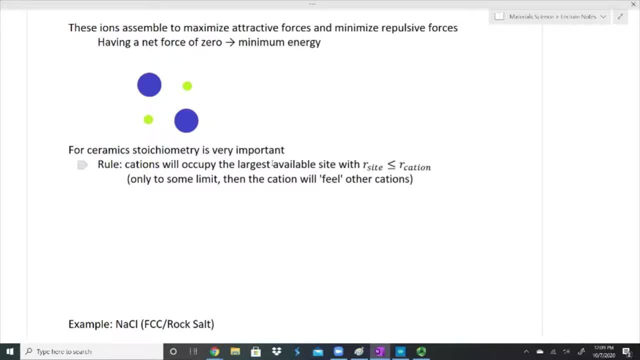 using are going to show that the charges are going to equal out. Sorry, Because we're dealing with charges here. we need to make sure that our positive and negatives equal out. The way they bond is going to work and everything We can't have a charged crystal, The crystal. 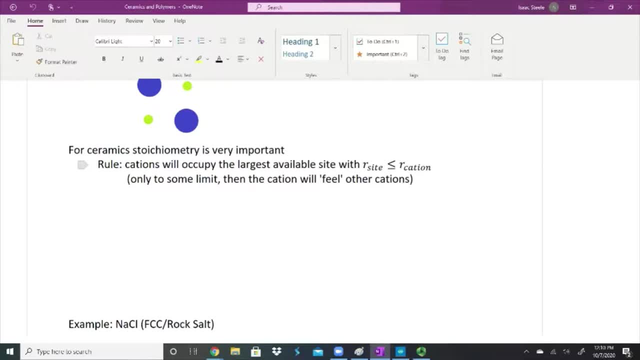 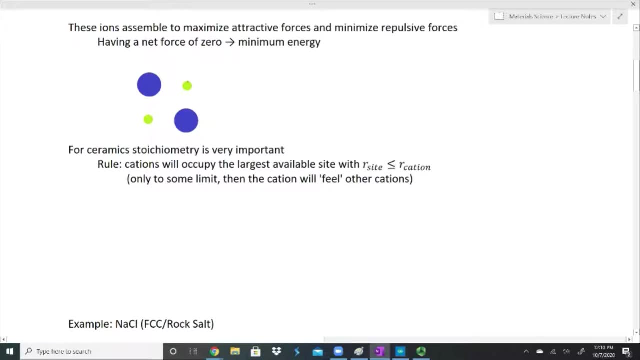 itself has to be neutrally charged. Sorry about that, for just I'm going to step back here. I want to talk about how these are going to assemble real quick. The cations and anions are going to be attracted to each other. These are going to want to pull together. 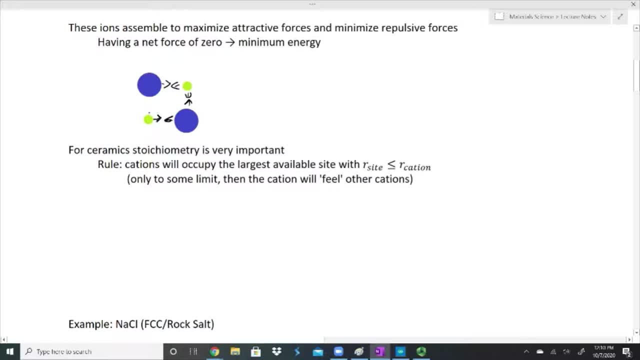 Okay. Also, what's going to happen is, as they pull together, these two blue ones here which have the same charge, are going to start repelling. They're not going to want to get so close. Also, the green ones are going to be getting closer together and they're going to try. 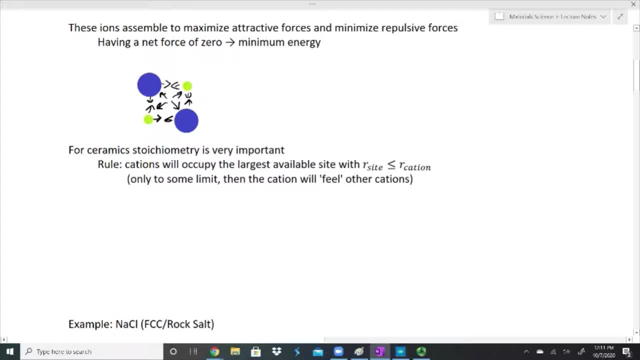 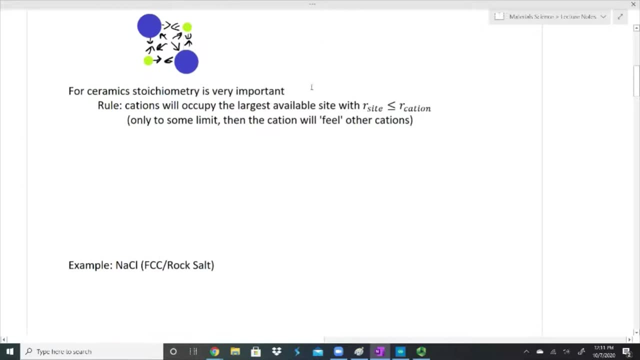 to repel. It's kind of this dance between where do we want to sit? and this is just in two dimensions. In three dimensions it's going to be quite a bit different. There's a lot more going on there. I do have this rule, a little bit about the stoichiometry and some other things We're 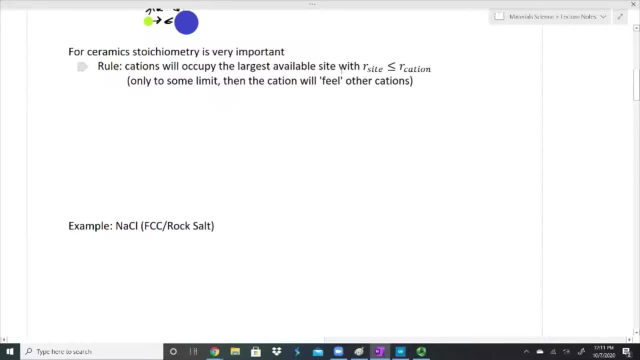 going to say that the cations are going to occupy the largest available site We have, that the radius of the site is going to be equal or less than the radius of the cation. This is only going to be up to some limit. This happens because they're going to start. 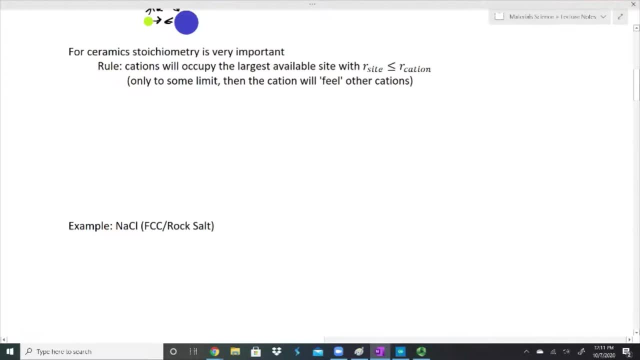 feeling each other. All right. Let me draw this out because that in and of itself might not make as much sense. I'm going to have a big red circle be my anion, and I'm going to make a small green circle. 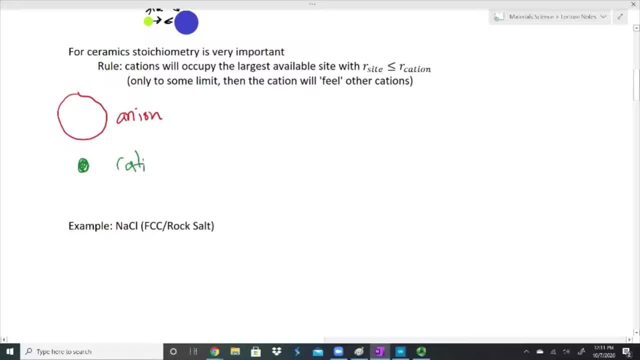 be my cation. All right, If I have my cation here and if I have my anions come in and they're too big, All right, Let's say that they are too big. Keep hitting the wrong button here. All right, I'm going to actually draw my anions first to make sure that this. 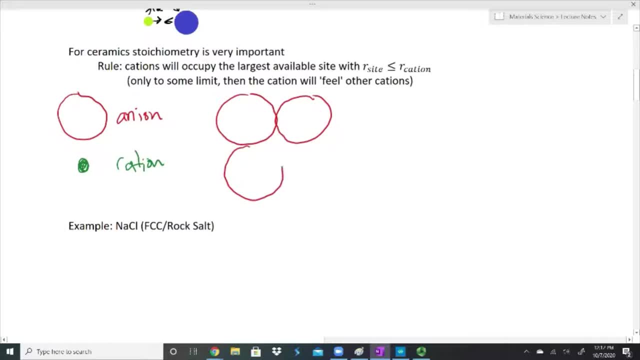 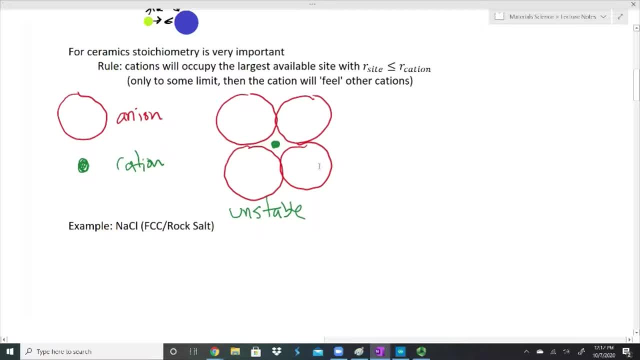 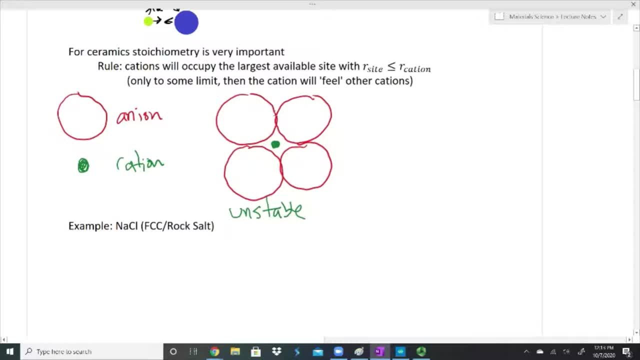 and they're the same charge and so they're not going to want to be attracted to each other. so why would they want to attract, to touch, if they can't get very close to the cation? we can have a different picture. let's say that i have a larger cation and or smaller anions. 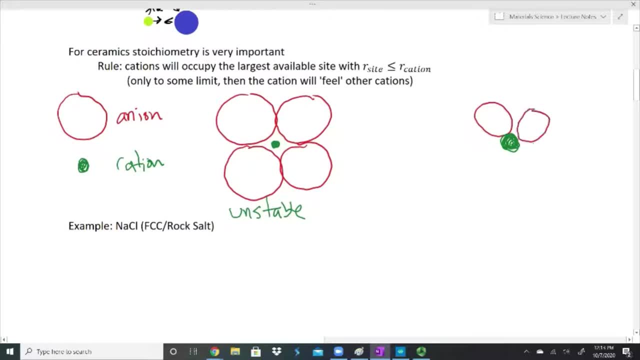 and so i can have a larger cation and i can have a larger cation and i can have a larger cation. we would say that this one is stable. the charges: everything's happy. positive is only touching negative charge things. there's a gap between like charges. if i were to continue drawing this out, i would have 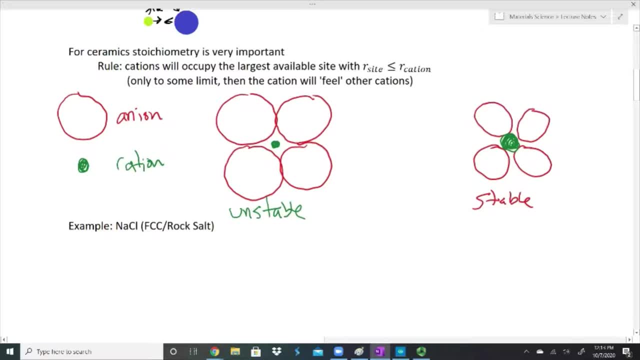 more cations, filling in these gaps with more anions state spaced plenty away. there is going to be a spot right in the middle that we're going to call the stability limit, and the stability limit is where we go from stable to unstable. basically, let's say that these charges are: are these: 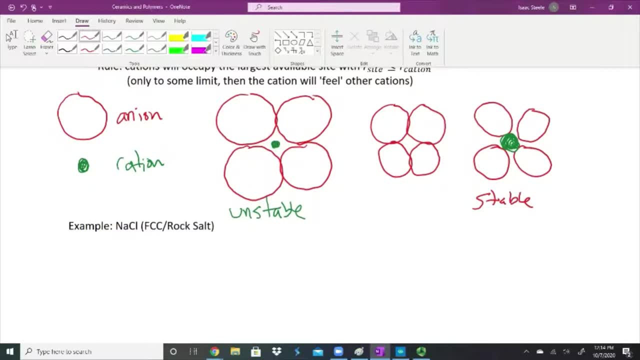 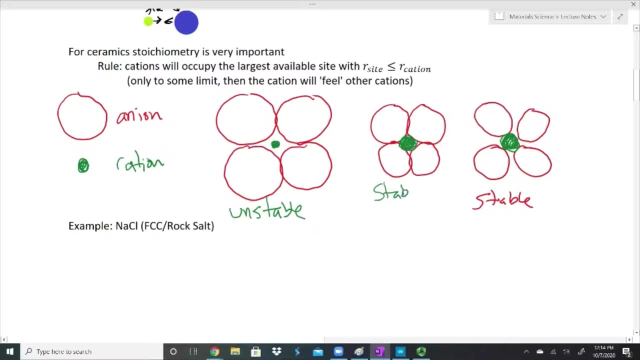 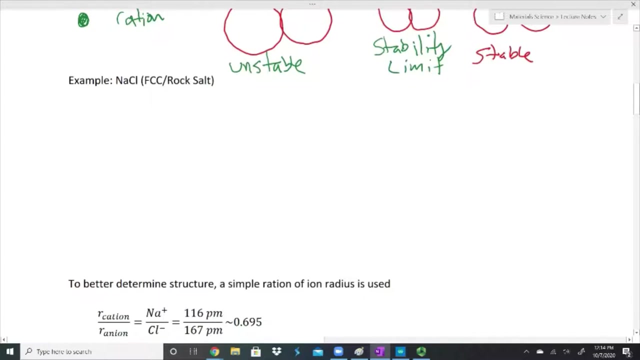 equally charged. ions are actually touching each other. the anions are touching, but it's also touching the cation again and it's actually taking the cations and getting the charge to fit in here. so again, that's a later time stamp period of wait. oh oh. 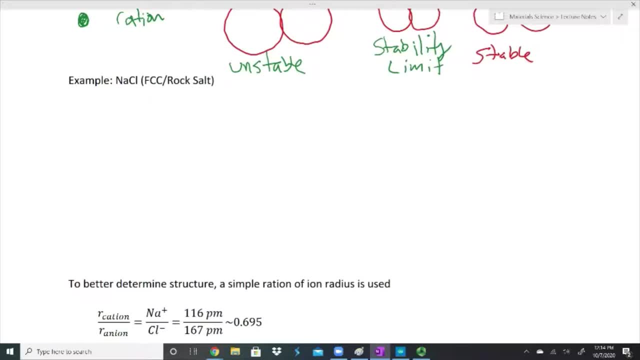 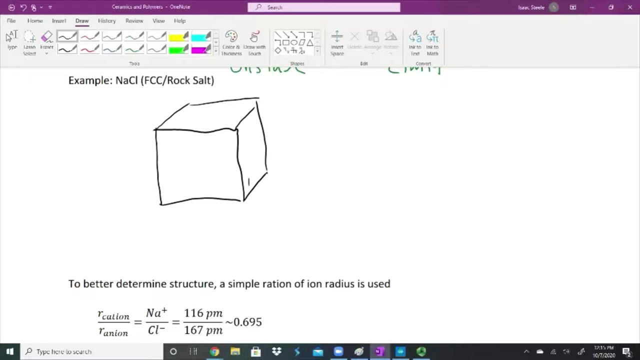 oh, that's okay. cubic: it's got a rock-salt structure, and I'm gonna try to draw this as carefully as possible. now, remember a face centered cubic: it's going to have a an atom on any given a face, and so what we want to look at here is- I'm actually going to draw this two ways. 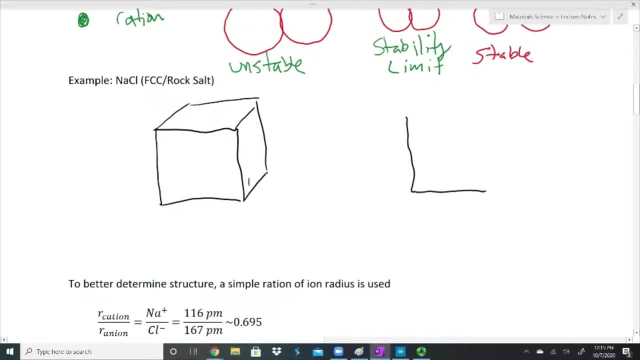 I'm going to go ahead and draw the second one really quick. there are two ways to think about this, so I could say that it's going to do this. I could say that I have. it doesn't matter which one this one is, I have the red one, let's. 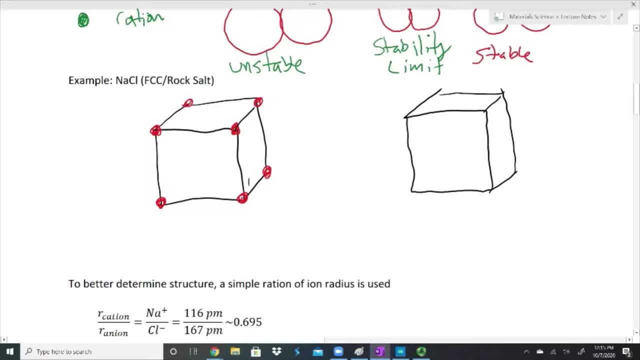 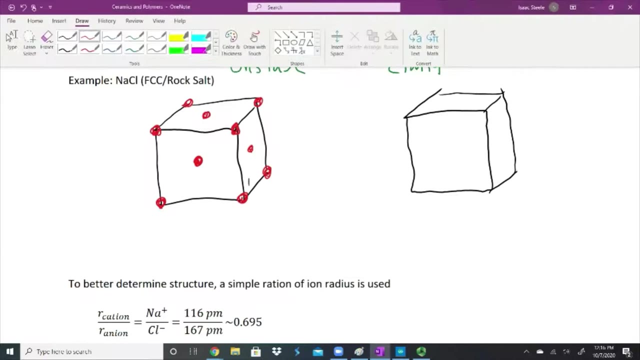 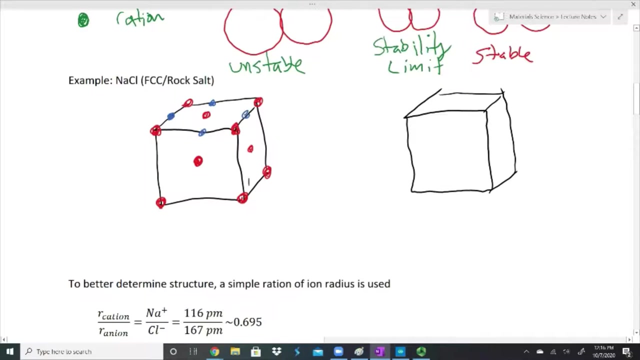 say: that's my sodium and I'm gonna have that on my face as well, because this is face centered cubic. so where then are my chlorine is going to be chlorines I'm gonna put on my edges. so initially I said it was face centered cubic and it. 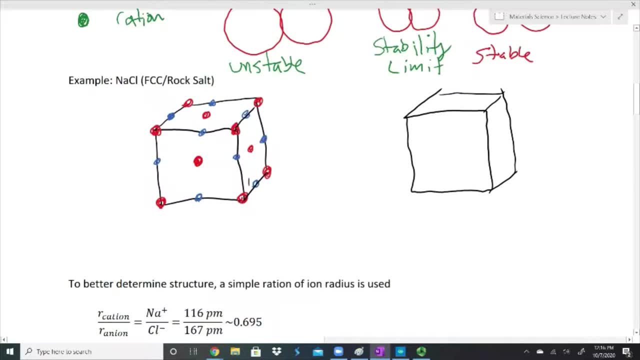 looked like face centered until I started adding in these blue ones here and now it doesn't really look like face centered- cubic, it looks like it's more. now I'm going to jump over to this other one, really quick, this other picture that I'm going to draw. we'll talk about the. 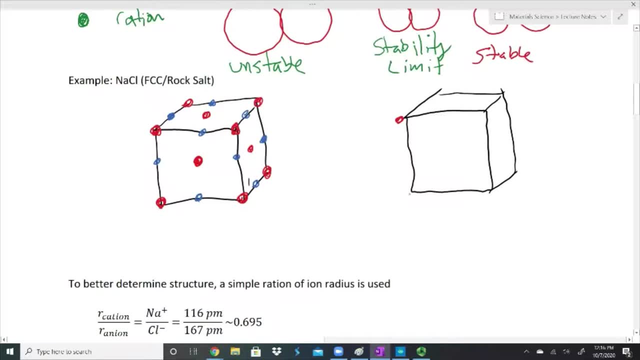 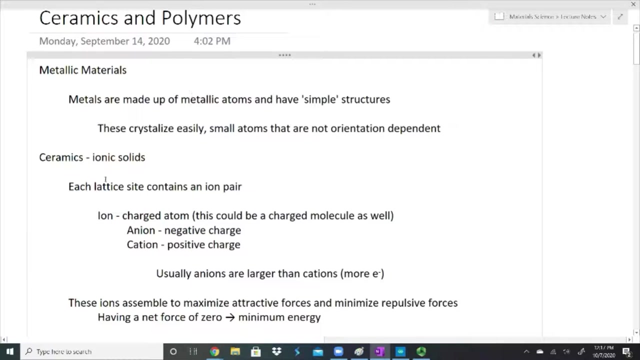 second picture. first, I'm going to just off to the side of each corner. I'm going to put my sodium- you put my chlorine- right at the exact same spot, or at least right next to it, and so when we talk about- and if I scroll up to the top, see where is it- each lattice. 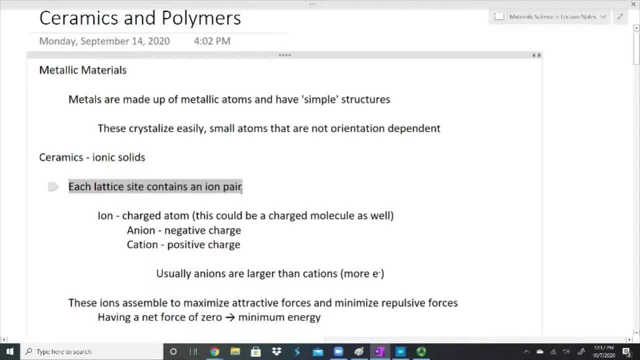 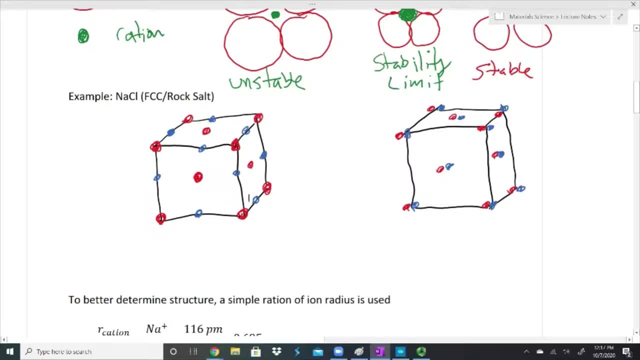 site contains an ion pair, and that's the picture that I drew here. so each lattice site, so this corner, has an ion pair, this corner has an ion pair, each face has an ion pair. now it's- it's a easy way to mention- that we basically have to have pairs so that we have neutral charges. when we talk about 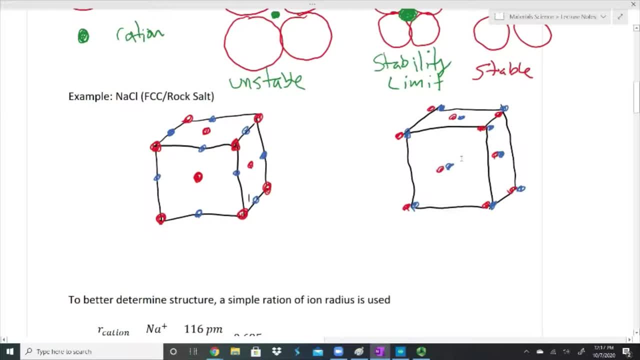 ceramics when we talk about ionic materials, but in reality we know that they're not gonna be nice and spaced out this way. so what actually is happening is a picture that is closer to what we have here, and in this picture i have a positively charged ion on the corner. 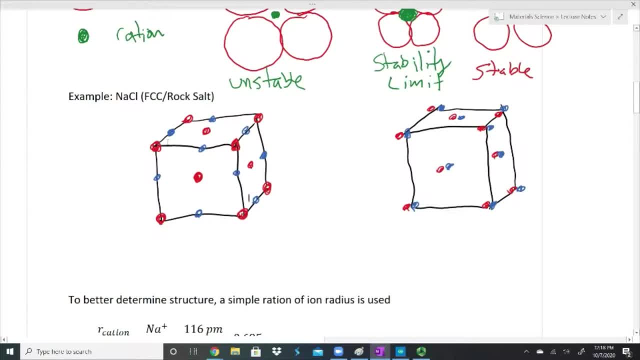 and it's negatively charged ion, it's pair. we've bumped over into the middle so that it's equidistant between these two positive charges. so what i'm really done here is, if i wanted to, i could extend out my unit cell just a little bit, just just a half unit out. 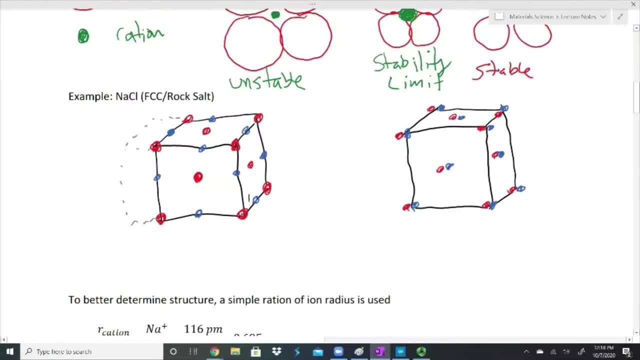 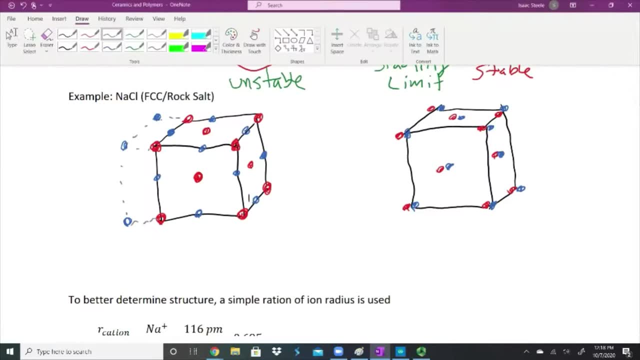 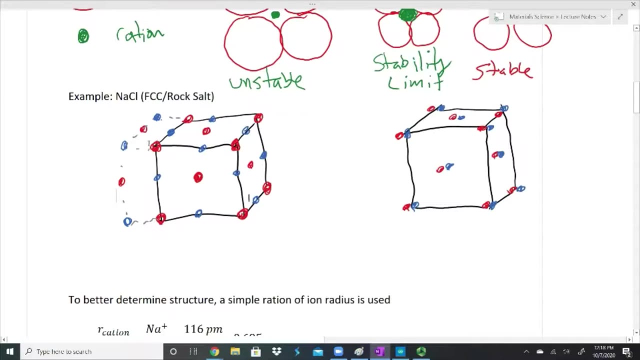 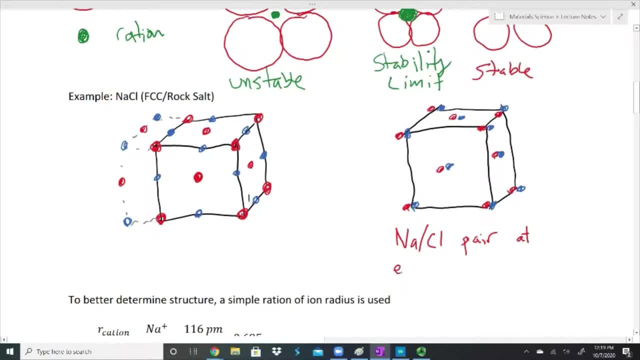 um at each lattice site. but what it really is doing and what it really looks like is we have two fcc superimposed lattices that are shifted just half a unit over. so if we kind of just ignore, let's ignore the blue one. so we're going to take the blue one and we're going to take the blue and then 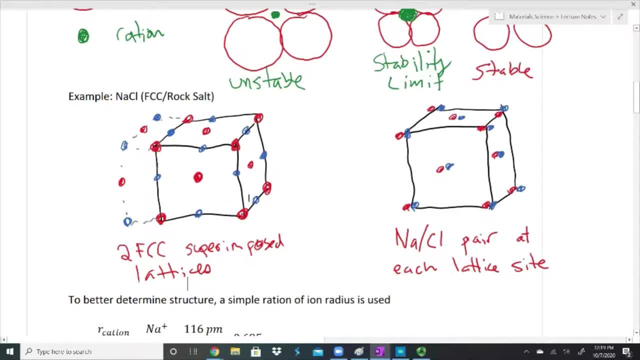 for now, If we just ignore the blue dots- and I look at this original one, I have an FCC, I have red at each corner and I have a red at each face. If I then ignore the red ones and I look at my dotted line box, here we have at each corner, we have a blue and we have a blue at each face as 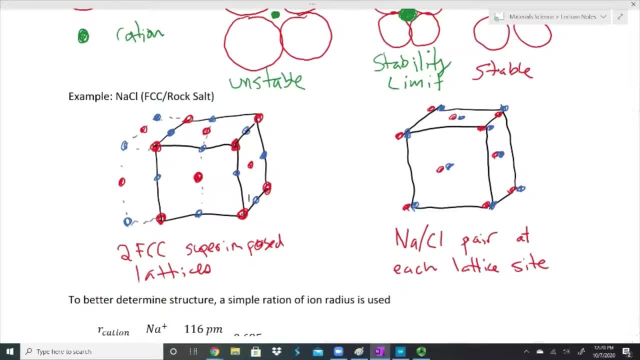 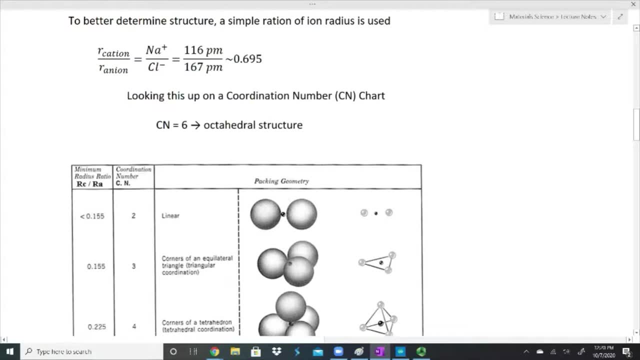 well, So we basically just have two superimposed lattices. All right, so what can we do Mathematically? what we can do is to determine this structure a little bit. better is, we can just take a simple ratio of the ion radiuses that are used, And so we do. the cation radius divided by 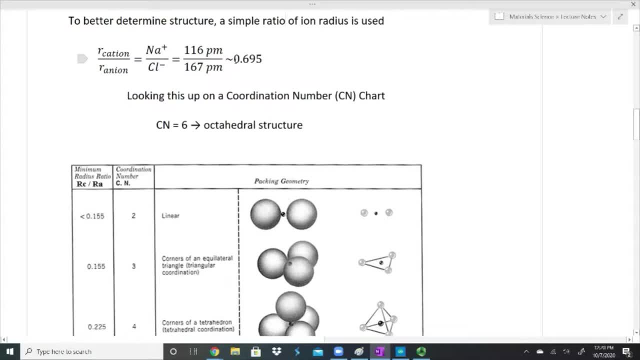 the anion radius And we're going to get some ratio. Now be very, very, very, very careful here. Make sure you are using radius of the cation and anion. They're going to be significantly different than the radius for just an atom that is neutrally charged. So make sure that you are getting the cation and 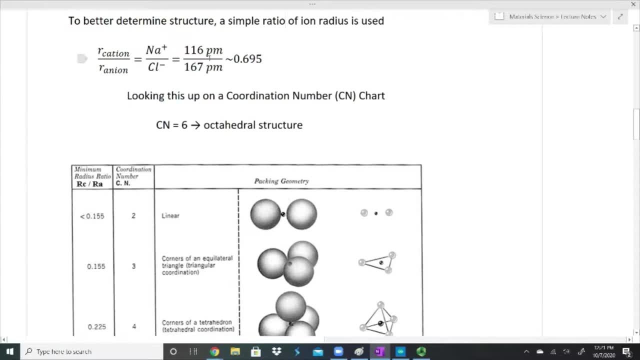 anion radiuses when you plug this in. I looked this up and, depending on the chart, of course, the numbers can be slightly different. I went ahead and plugged those in And I got about 0.695 for my radius. What I can do, then, is I can go to this chart below and I have 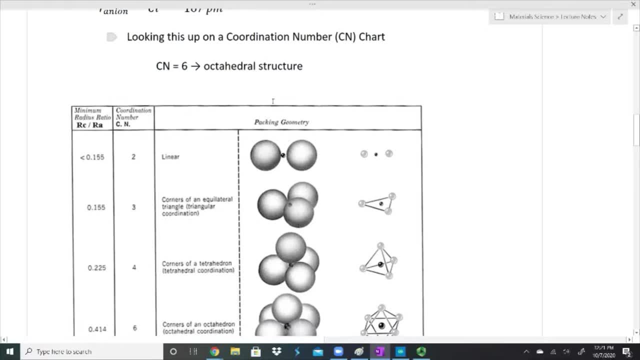 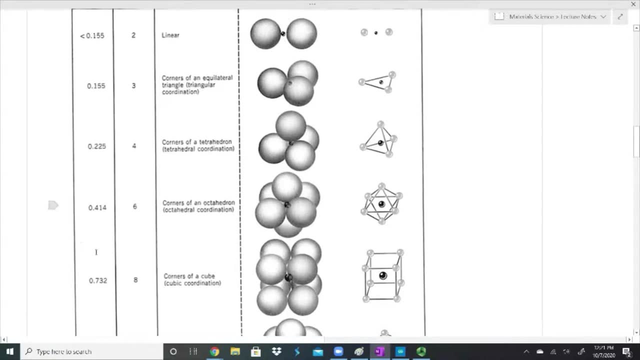 this coordination number chart And I'm going to try to find where this number fits in. And this number fits in in between here, So it's in between 0.414 and 0.732.. And so what I have here is I have a coordination number And I'm going to try to find where this number fits in. 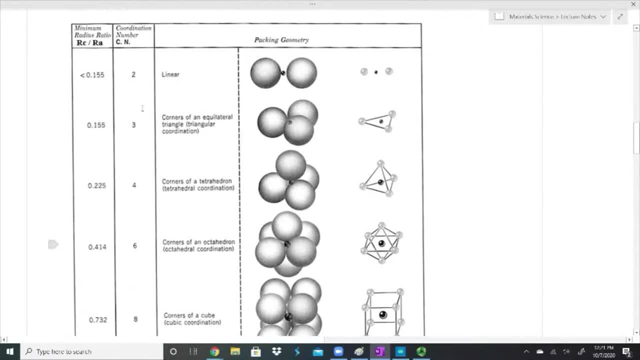 This is a coordination number of six. Now, what the coordination number really is saying is how many nearest neighbors does it have that are of an opposite charge? And so if it falls between the range of 0.414 and 0.732, it's going to have six nearest neighbors of an opposite charge. 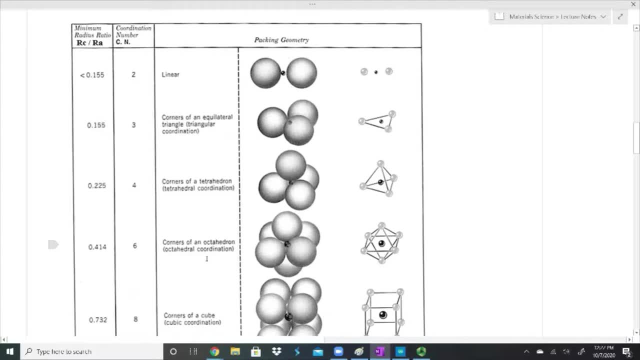 And it's going to form an octahedral type pattern, And so this is what it would end up looking like. And then, of course, I could repeat this over and over again, and over and over again, like we do with our other crystal structures. really quickly we're going to. 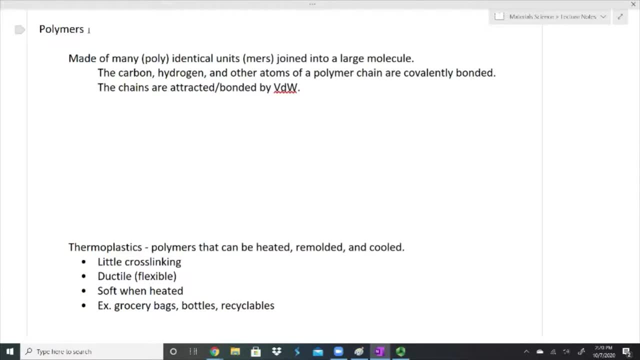 go through polymers now. polymers. there's a lot of stuff here and we are going to go through it really quickly. we can talk about it more if you want to get into polymers, but we're really just going to hit some things. we're going to go through this really quick and there's a ton of stuff that 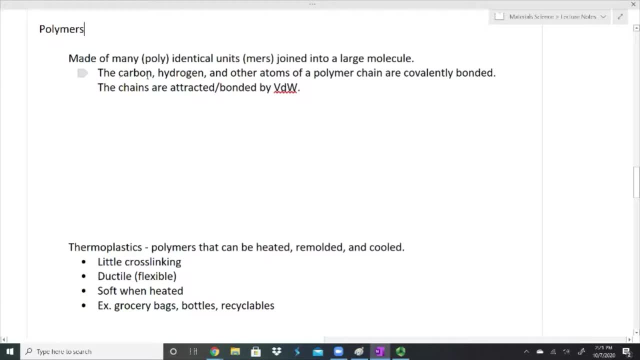 we're going to talk about. so, first off, polymers mean many units, and these many units are joined together into a large molecule. there are carbon, usually hydrogen, and then there can be other atoms, and they're all covalently bonded together into these long chains. and these long chains are: 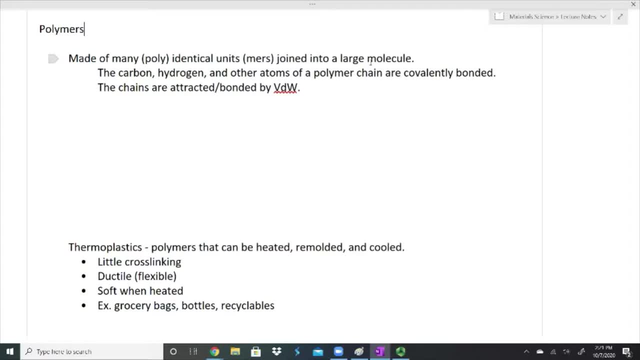 then attracted together from the sides by van der waals. so really quickly, if i were to just sketch, i would have a bunch of stuff happening in this reading part of. i would have a bunch of stuff happening in this reading part of. i would have a bunch of stuff happening in this reading part of. 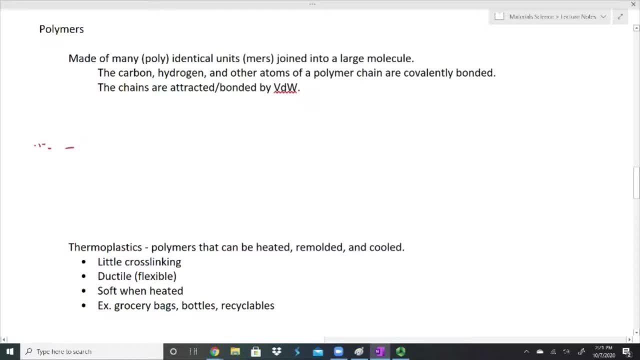 over here and then I'm just drawing a small segment of this long polymer chain. I have a carbon, it's bound to a carbon, it's bound to a carbon, it's bound to a carbon, and so forth, and it just keeps happening like that. what we're gonna see. 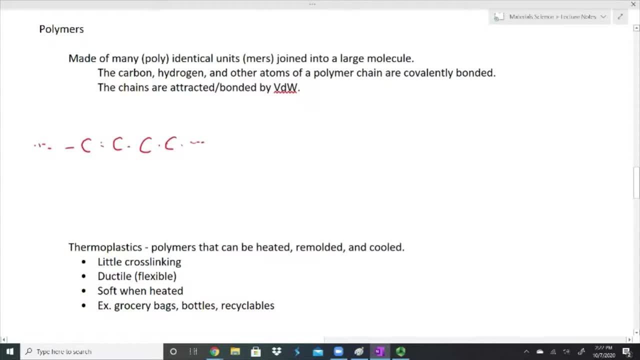 though, is off to the side because, remember, carbon is going to be able to have multiple bonds. in this case, it's gonna have four bonds. two of them are used up just by bonding to neighboring carbons, but the other bonds are going to be something else, and right now I'm just gonna put an R here. 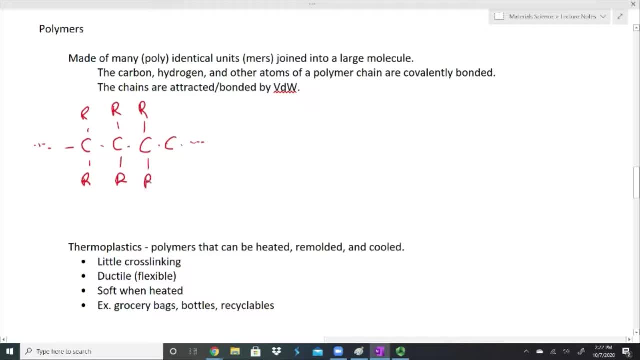 but they can be really any molecule or any atom that it can bond to. sometimes they're simply just a hydrogen. so this is one way to do it. it's a two dimensional drawing of what's happening here. there's another way to do it, and that is: we can just I'm gonna try to make those a little bit more. 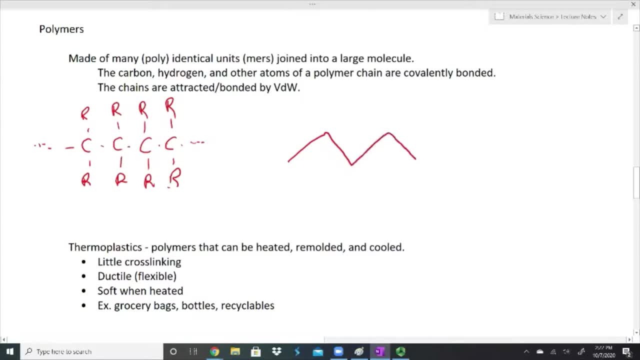 crisp, nice corners and what it is is at the end points. so on both ends and add these, these peaks and valleys at the corners, what it is is there's a carbon sitting at each one of those. it's just shorthand, so really there's a carbon right here. 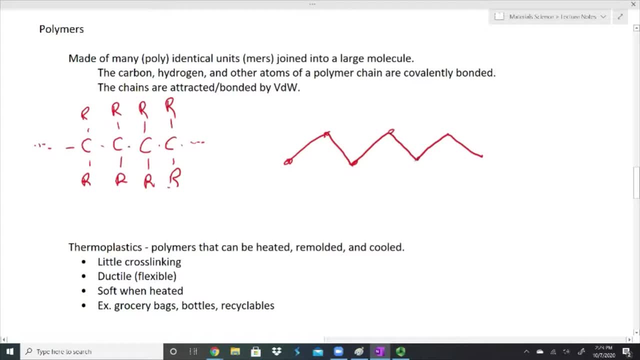 there's a carbon right here. there's a carbon here here. that way, I don't have to draw out all my sees. also, shorthand is, if they're simply just hydrogens that are sitting attached to each carbon, i can just leave it blank. there's nothing else i have to do. we just understand that there are going to be two. 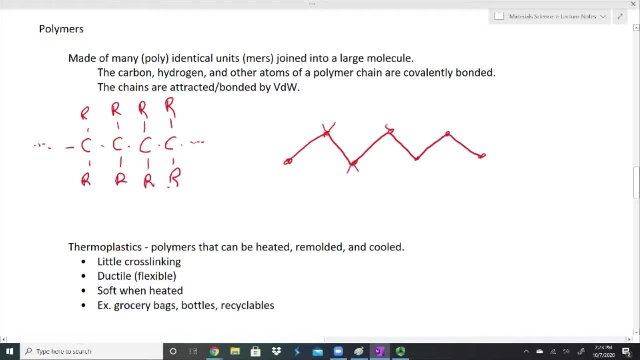 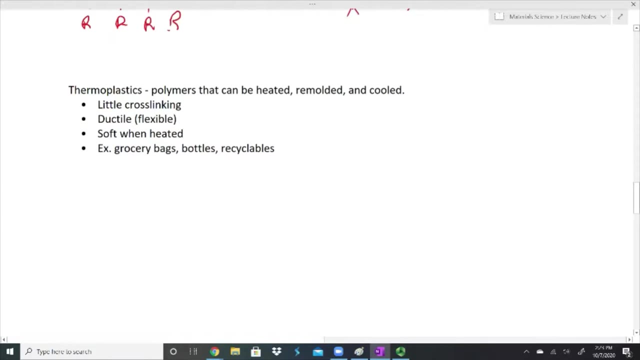 hydrogens there, but there could be other things bonded here that are maybe not hydrogens, and so that's something to keep in mind as well. so these are attracted together. we're going to go through a couple different ways to do that. number one: we have thermal plastics. thermal plastics are 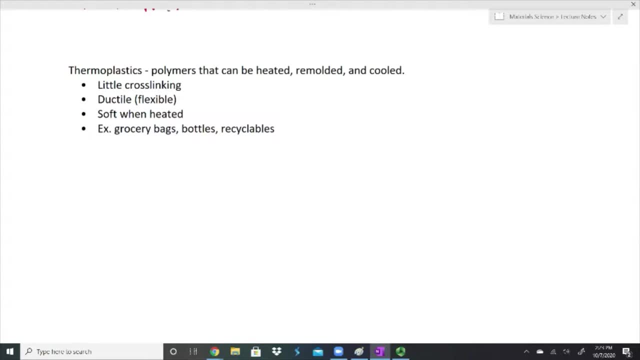 polymers that can be heated, reheated, remolded, cooled multiple times. there's very little cross-linking, which we'll get to in just a second. properties of this is they're ductile, they're flexible and they get soft when heated. examples of this is normally things that we think about. 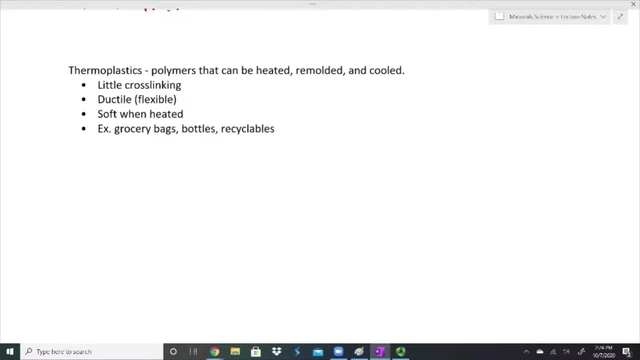 when we talk about plastic grocery bags, bottles, things that you can recycle, and so if i have a polymer chain and i have another polymer chain that nears it, gets by it because, again, these are just long one-dimensional molecules. for the most part they're. they're really long in one. 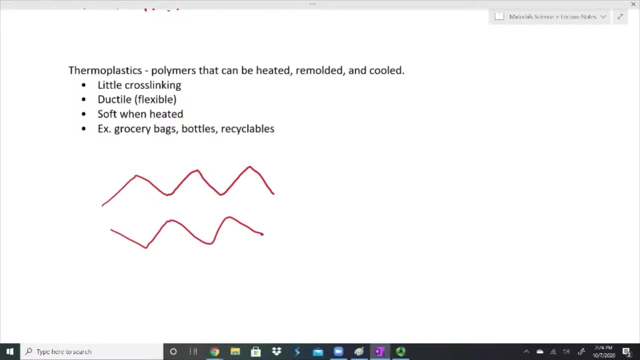 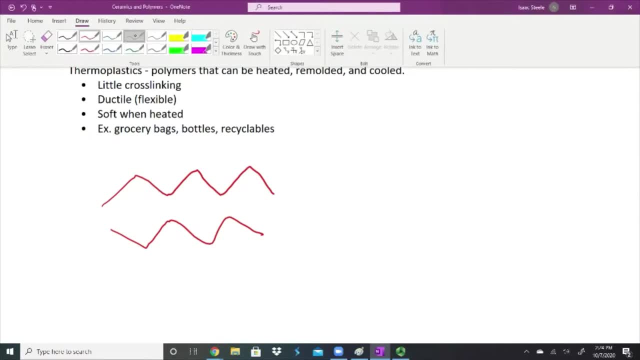 very good, and it's in an earth, vamos. so here, what we're going to be doing to do is: how is it going to move back about and start reflecting back in on itself? there's going to be some attraction here and these small structures in the middle. 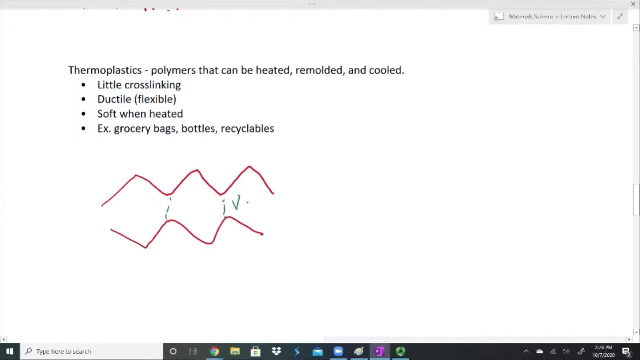 attractions are going to be van der waals. this is a linear chain, linear attraction. basically, we have these long linear chains and they're attracted to each other. we could have a branched polymer and a branched polymer. polymer is very similar, but what I have is maybe something where I have a branch. 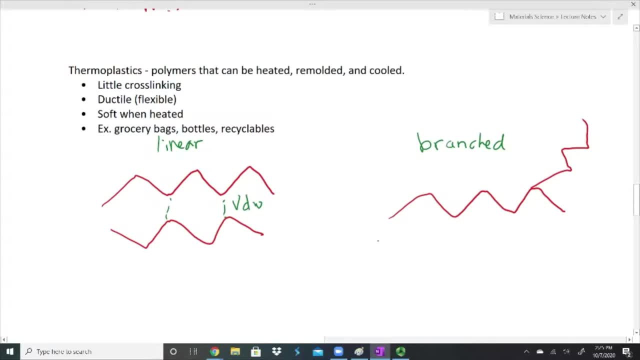 and another polymer comes off of it, and again I could have another one over here and maybe it has some branch as well. so there's some branching going on. in this case it's still going to be held together with the van der Waals forces as it gets. 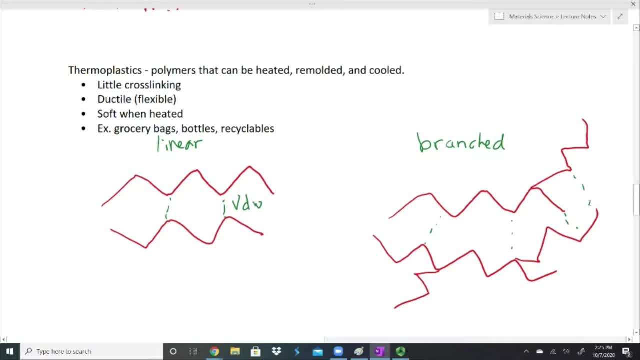 close to other polymer chains. so some examples of this would be: if you've ever looked at some plastics, if you've ever recycled some plastics, maybe you've heard of HD PE, that is, high-density polyethylene, and that's what the hd is for is high density, the branched one. an example of that would be l d. 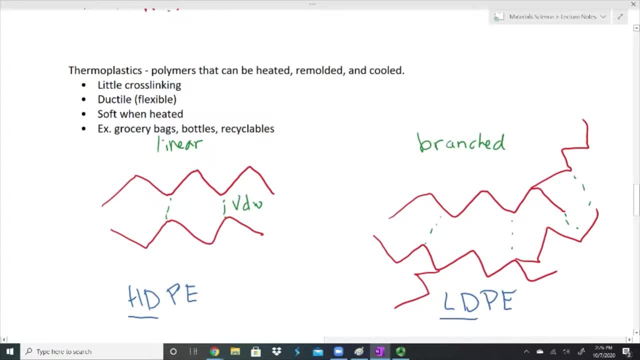 p e, which is low density polyethylene. basically they're the exact same polymer, except for one is more densely packed together, and the reason it's more densely packed is in the linear picture. i can get these a lot closer together because these long linear chains can be. 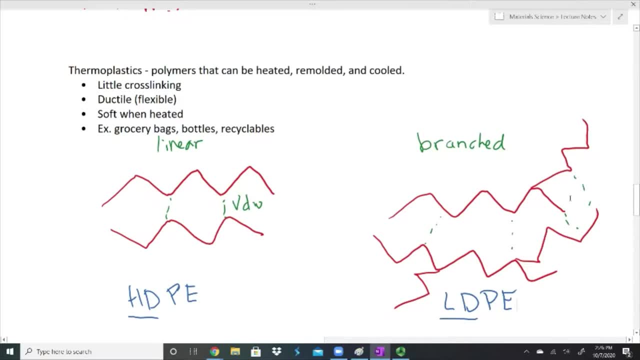 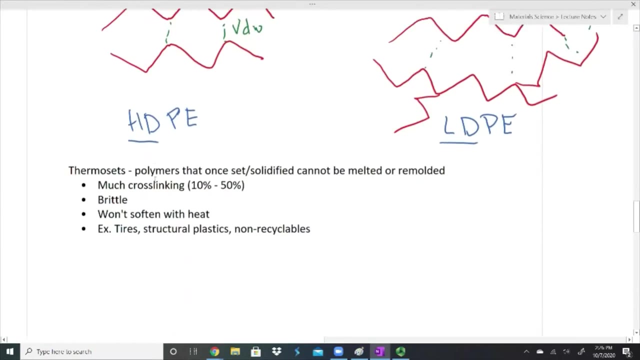 uh, and can squish together a little bit more. if things are branched, it's kind of pushing itself apart. i have more gaps and so if i have a branched polyethylene polymer it's going to be a lower density than if i have a linear polyethylene polymer. we'll talk about thermal sets really. 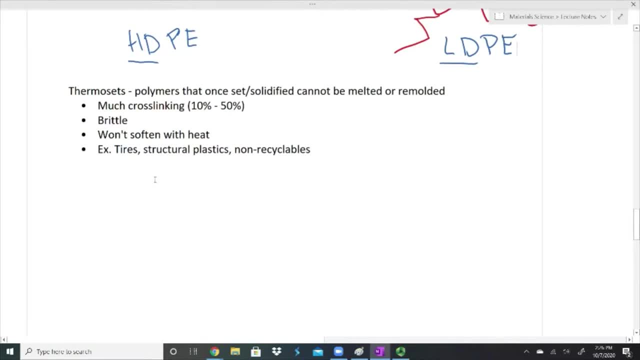 quick thermal sets are polymers that once they set, once they've solidified, they can't be melted or remolded. there's a lot of cross-linking that happens in these polyethylene polymers and this is sort of where it happens and this is where we're going to talk about what cross-linking. 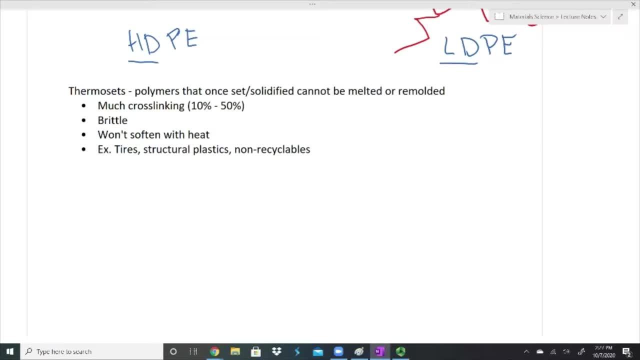 is they tend to be brittle, they don't soften with heat, and some examples would be things like tires, structural plastics or non-recyclable plastics- and again, they're non-recyclable because you can't. you can't heat them up and remold them. there are some things you can do. we don't. 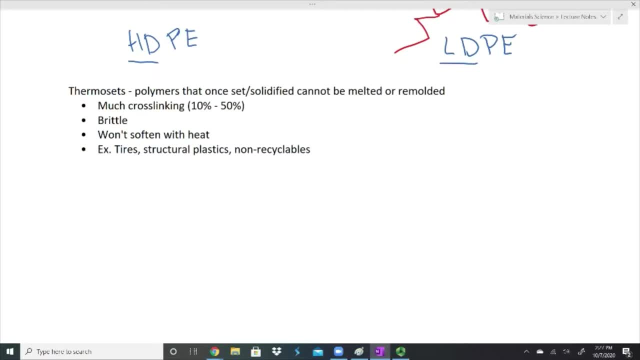 necessarily consider recycling, but if you want to get rid of it and you want to use it for another purpose instead of just being waste, do something like shred it or grind it down and use it for filler somewhere. so what it is is, let's say, i have a polymer chain and another polymer chain that comes into it or comes near it. 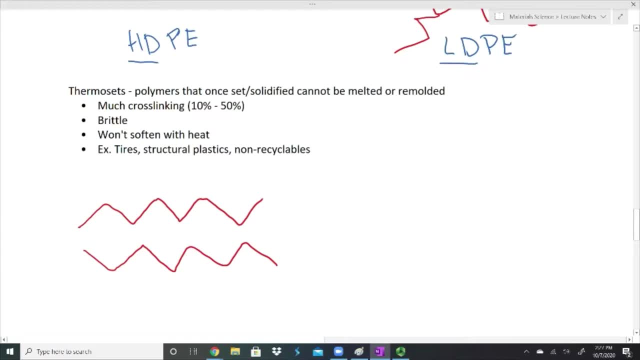 instead of them just being attracted with the van der waals forces. what i can do is i can add some type of catalyst in there, and a lot of times these are epoxies, they're resins, and you add some type of additive to harden it and to cause this reaction to happen. 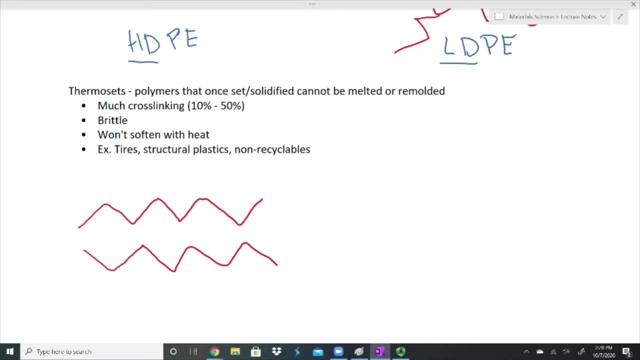 and a lot of times when you use epoxies, they actually get warm or you can see some type of steamish smoke, something coming off of it, and what's happening is it's actually changing the chemical structure. we're actually forming new covalent bonds. these are covalent bonds, not 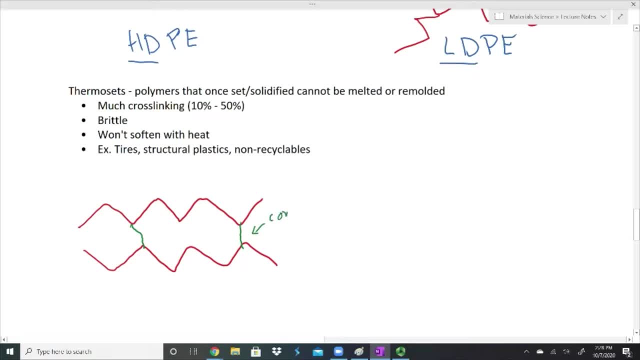 van der waals bonds. they're actually covalent bonds. there are going to still be some um some van der waals forces wherever the covalent bonds don't happen. but these are much, much stronger because we have additional covalent bonds. but it also makes them brittle because we can't slide them like we could with the van der waals. 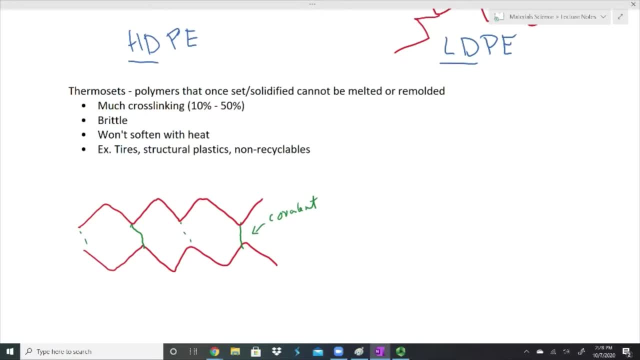 it also means that we- this is the reason we- can't soften them with heat. i can't add some heat and then magically have these new covalent bonds just disappear because i decided to reheat it. once those covalent bonds are made, they're as strong as as the other covalent bonds. 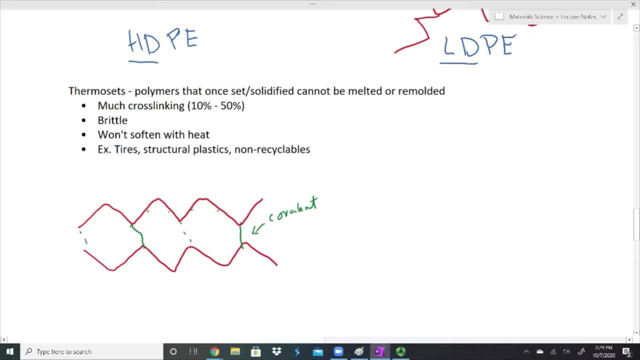 in my original polymer and i can't you know, break just the the new bonds and leave the old ones there. this one would be a cross-linked material, and the more cross-linking i get, i end up eventually getting a networked material, and all in. network material is one that has a significant number of cross-linking: um 100. 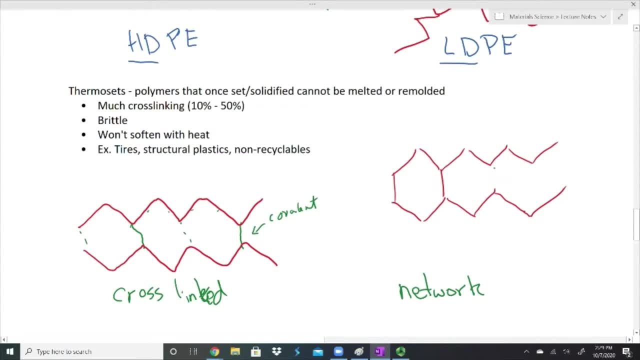 networked material would look something like this: where i get these um polymer chains together and i, that should look like that um, these these link together everywhere. it's completely networked together. this part should not be here, so that would be what a um, a complete network material. and so, again, the cross-linking are the 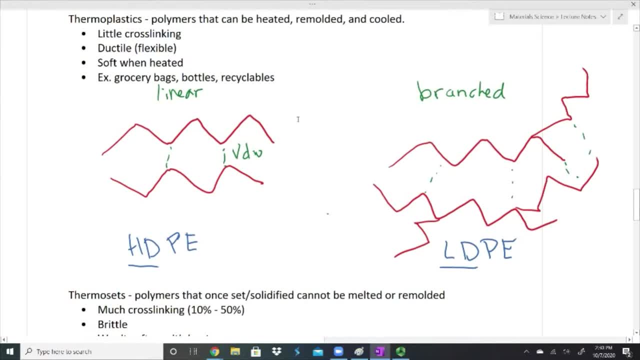 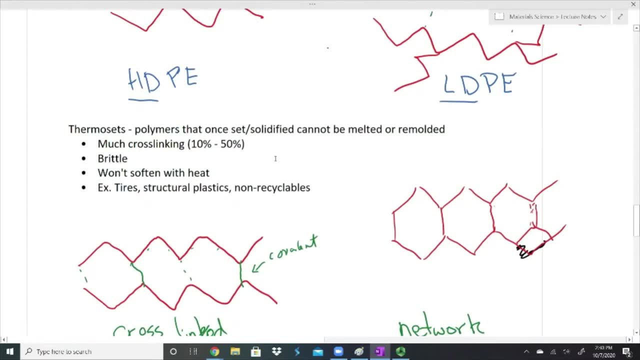 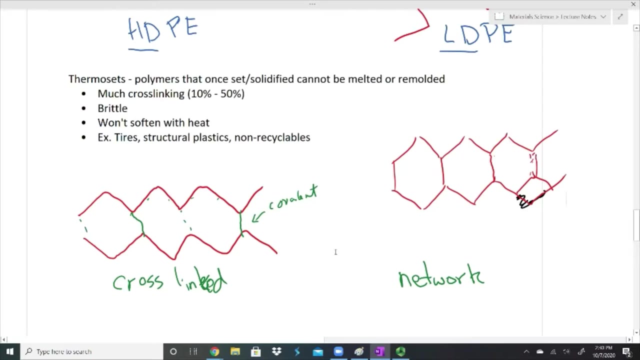 new covalent bonds that are formed. so if we go back up here, there is little to no cross-linking, it's all van der waals forces between these, uh, these, polymer chains, and with thermal sets, they, uh, we do form new bonds, which is why we can't recycle them or remelt them. 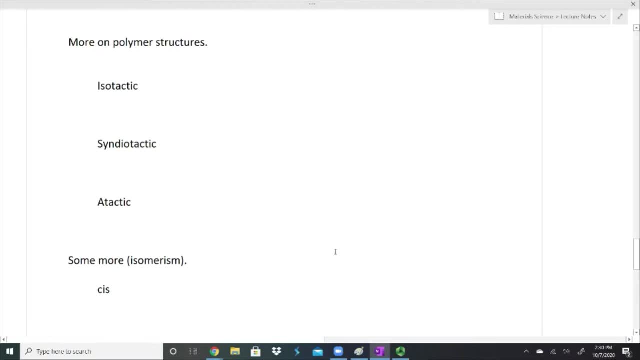 all right. so now we're going to even move a little bit quicker, because this there's a lot of information. more than anything, this is just going to show that we have so much going on here, but i'm really not going to spend the time to uh to go into detail on these things. 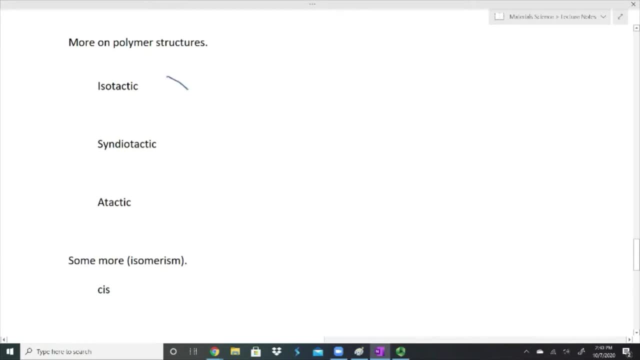 so we have isotactic. isotactic means that i have a polymer and my side groups. i'm going to have one side group that's coming out towards me and one that's going into the screen. one that's coming out and one that's going in, one that's coming out, one that's going in. 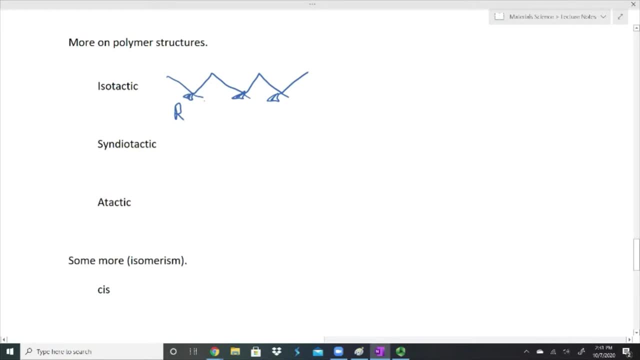 and what we have is we could have a molecule on one side and, let's say, a hydrogen on the other, and that pattern continues. and so if i was looking down this molecule, if i was walking down this entire molecule, like the molecule is a path on one side. 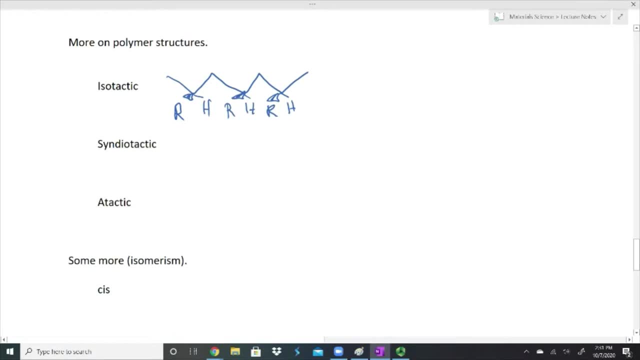 i would see all of my r's and on the other side i would see all of my h's. that's what isotactic means syndiotactic again, i'm going to have something coming in and something coming out on each one of these. in this case, they're going to flip-flop. i'm going to have an r and an h and then on this one, it's. 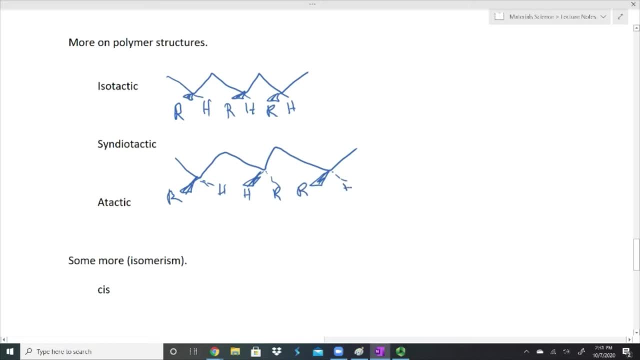 an h, then an r, r, then h, then h, then r. so if again, if i'm walking down this, I see my R on my right and an H on the left, I take a step to my next one and it's flip-flopped. 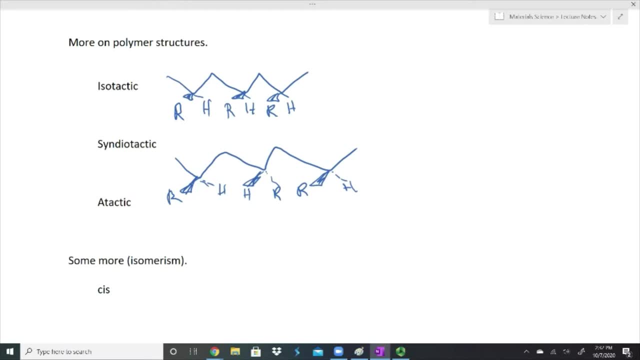 It's now an H and an R and then it's an R and an H. A tactic just means that it is random. I could have an R and an H, I could have an R and an H, Then I could have an H and an R. 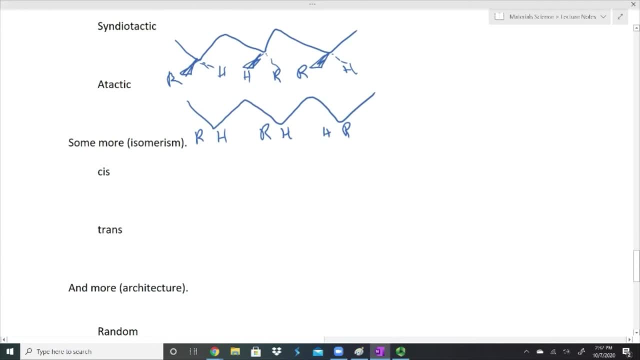 There really is no pattern along it. All right, even more stuff. We have some of what we call sys, and sys would look something like this: I would have my molecule coming in, I would have CH2, and it would come together. 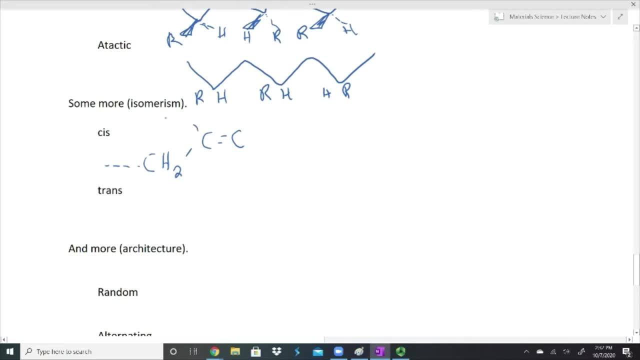 Let's say that I had this double-bonded carbon and up here I had a CH3.. Over here I would have my H and down here I would continue on with a CH2 and so forth. It might take you a while. 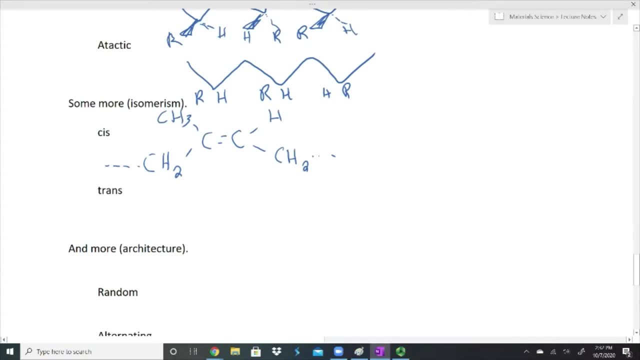 You might have to look at this on your own Again. I'm not getting anything. I'm not getting into all these little things, but I do want to show you these things. I'm going to draw my trans over here. That is sys. 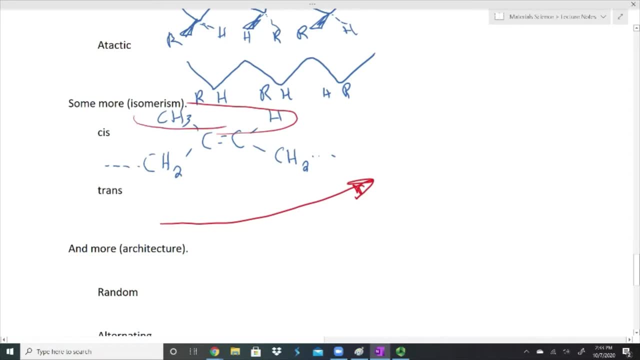 They're on the same side. These are both on the same side. With trans it actually jumps sides. If I draw this same picture- CH2,, C, C- and I have this same picture. I have this double-bonded carbon in the middle. 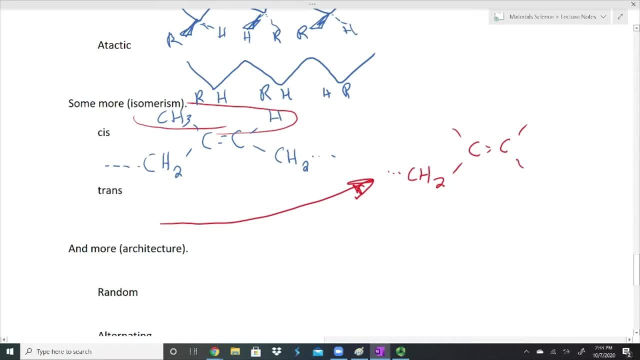 with these branches coming out and instead of my polymer chain, both being on the same side, it flops. My polymer chain moves over there and over here I am going to have my CH3,, let's say, and my H over here. 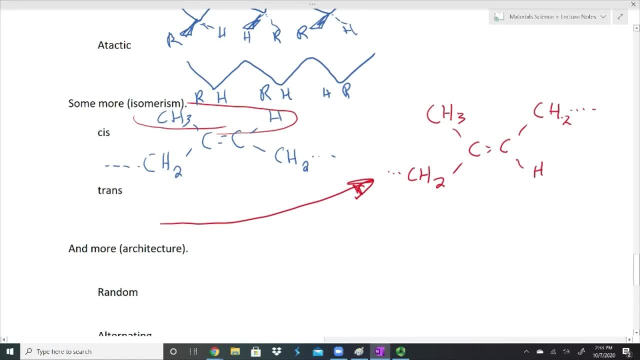 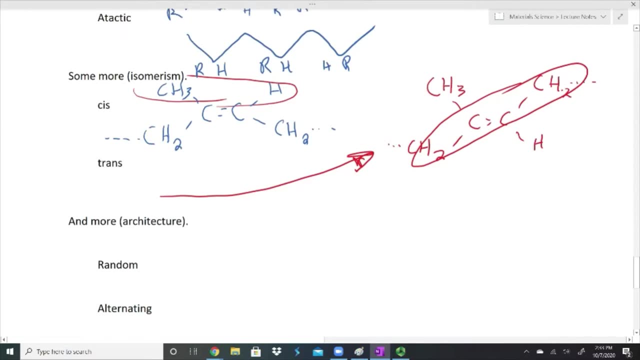 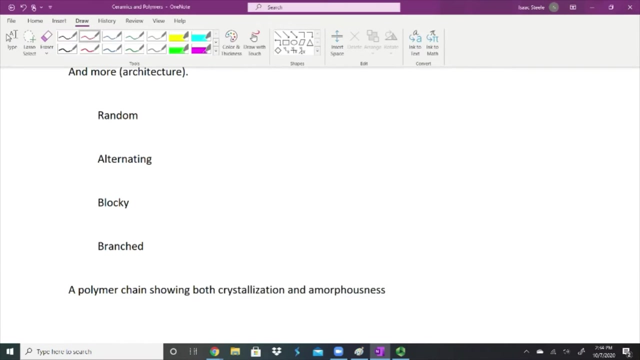 or whatever it happens to be. They really could be any type of thing attached, But this one, it goes across and that's trans. All right, Now we have even more things that we want to talk about. I could have blocks of. 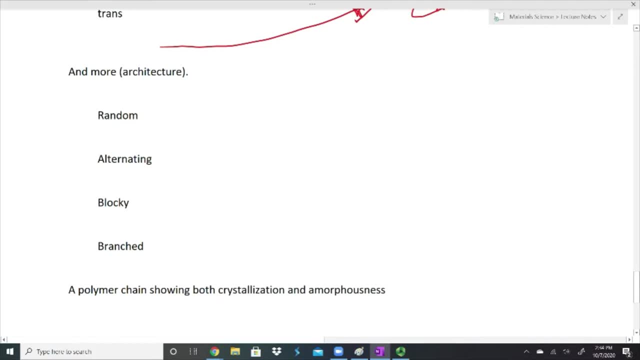 or sorry, I could look at my polymers and I could have kind of a random structure I could have, let's say, that each one of these circles is one of my MERS, one of my units of my, of my polymer. 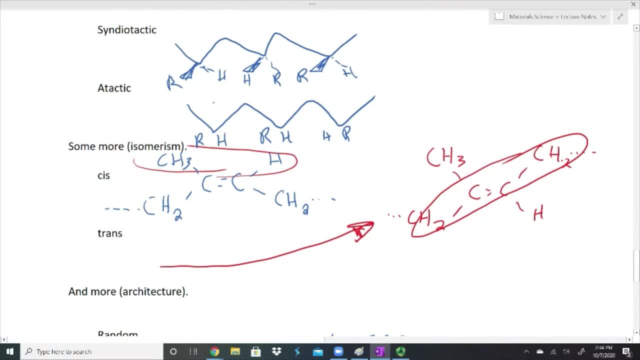 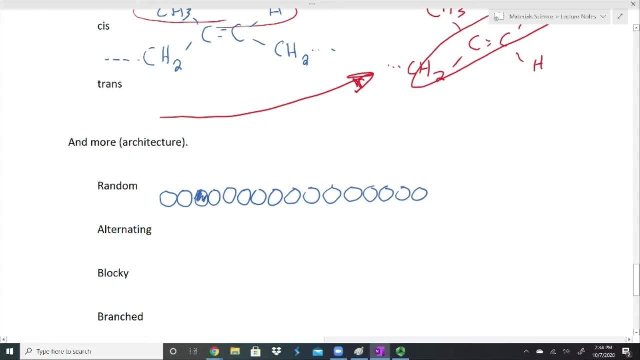 right, one of my these triangle-type shapes up here, So that is the circles, And what I could do is I could have something random where it changes for a while maybe into a slightly different chemical that's being attached and then it goes back. 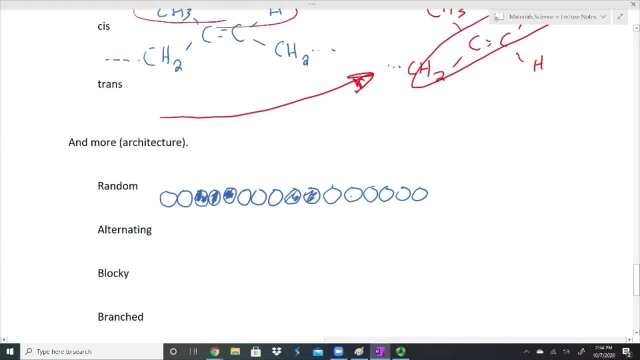 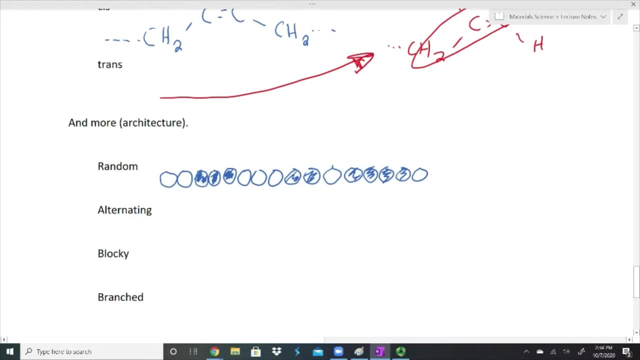 and then maybe a little bit more of something else, and it just kind of jumps back and forth between some. It kind of has this random structure. I could have alternatives. Let's say, for example, I could have alternating, and alternating I think sounds probably pretty standard. 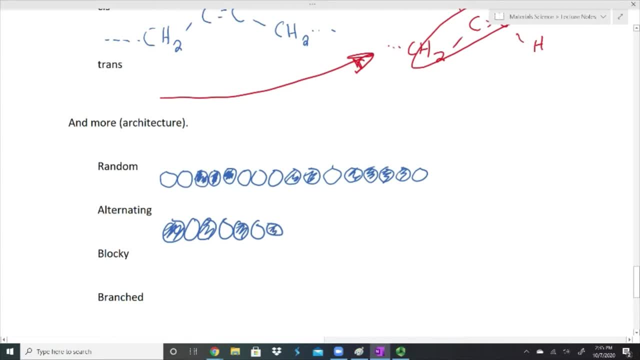 It just alternates between what my MER looks like, what that chemical unit looks like that's bonded together. I could have blocky, and blocky ones are where I have these large swaths of one type of polymer and it's all attached into one long structure. 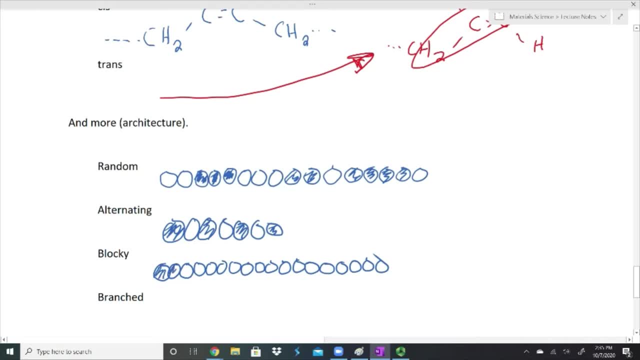 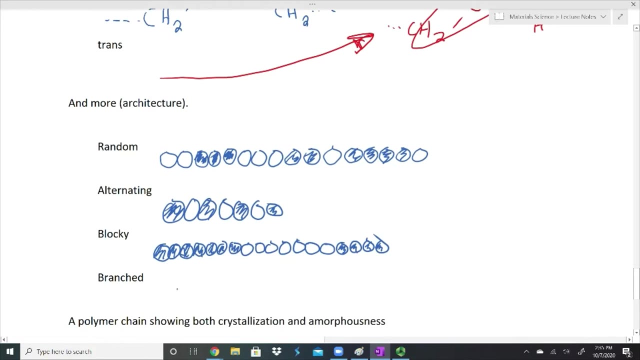 It's not a whole strand, but maybe for a while. I all have one kind and then I have another kind and then maybe it goes back, but I have these go in blocks. And lastly, we could talk about the branches again. 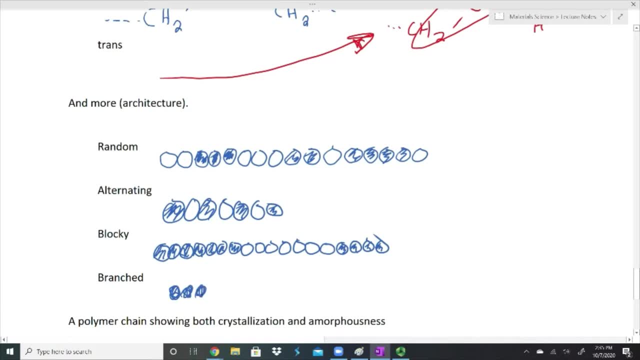 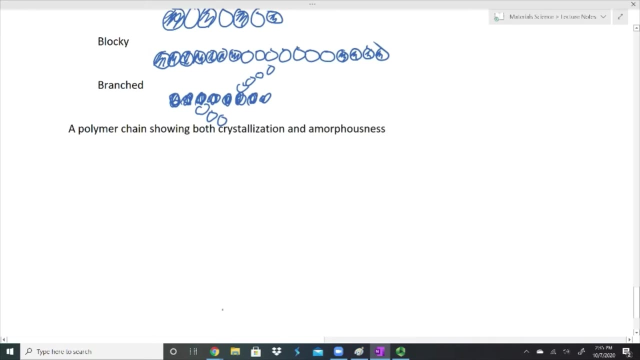 And what the branches could look like is. I could have all my backbone be one chemical structure and my branches could be a completely different chemical structure. So there's a lot of stuff going on here. Last thing that I wanted to show real quick is: 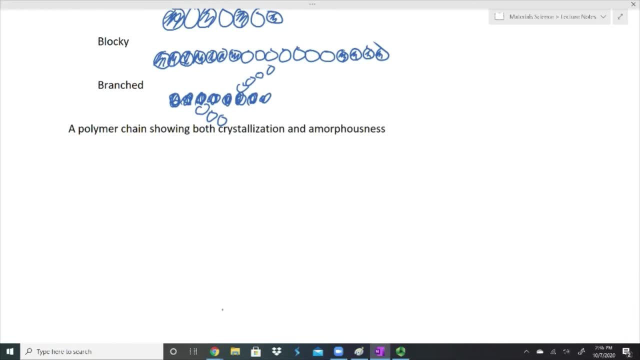 I wanted to show how a polymer chain crystallizes and how it's amorphous. If I just even have one polymer chain- and it's really really long- it can fold in on itself, And I'm going to draw this in two dimensions. 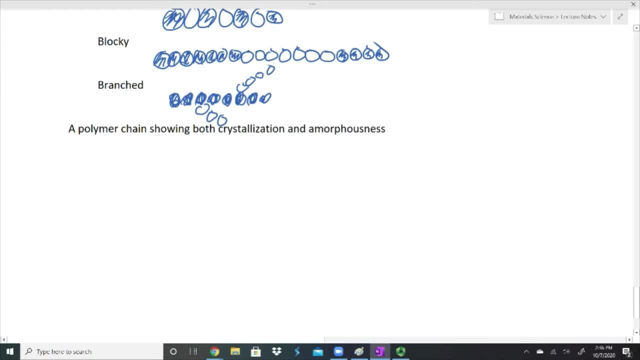 but remember it lives in a three-dimensional world And so if it were to crystallize, I could have these match up and it might even fold up on itself And these are really close together and they will crystallize. Now remember that, the way that it's attracted here. 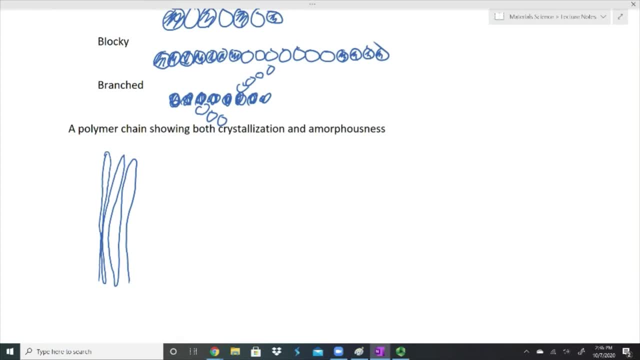 are van der Waals forces, but they are stacking together. It bends up in on itself, And so if we look at this middle section here- I didn't draw it necessarily super, super pretty, but you can see how these are stacked together- 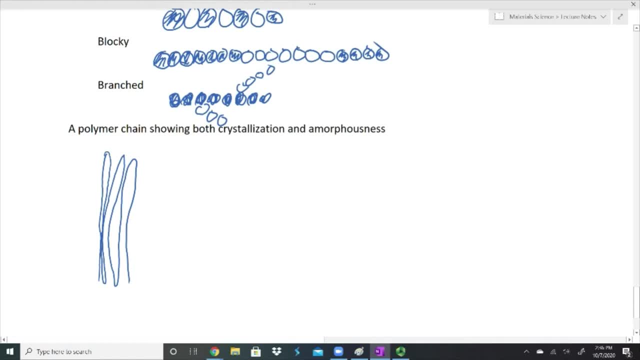 and it has some direction. It's very well oriented. Now, in the exact same polymer, it might stop crystallizing and it might start getting kind of crazy and be more amorphous, not have much of a structure at all, And so then it would be more amorphous. 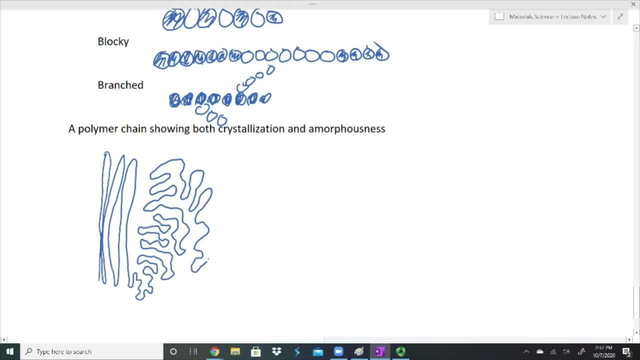 if it were folding in on itself like this, and then it might start crystallizing again over here. It can really do a lot of things. Polymers are very, very interesting. When we talk about polymers, we usually associate polymers with a molecular weight.